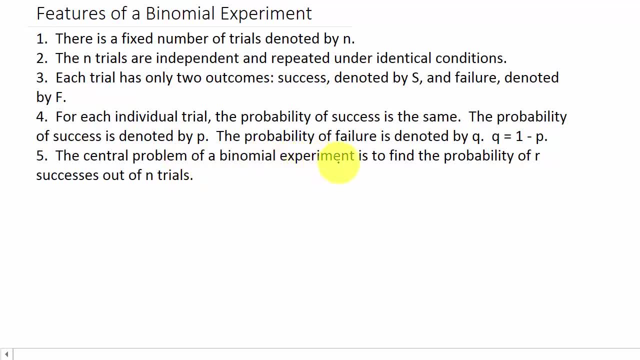 And the central problem of a binomial experiment is to find the probability of R Successes out of n trials, Okay, so there is a formula that you can use. So if, if we have the probability of R, Okay, and we have n trials, But we want to know the probability of R successes, The formula is: combination n choose R. 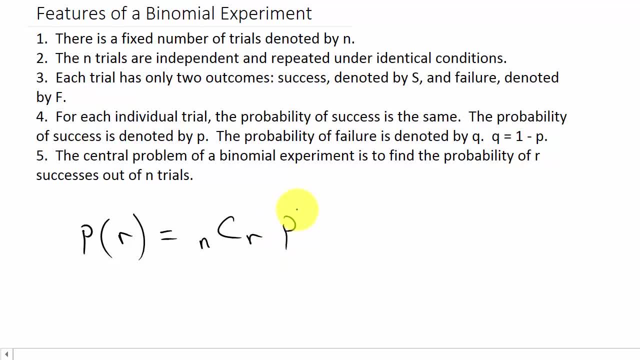 Times P, the probability of success raised to the R times Q, Which is the probability of a failure raised to the n minus R. Okay, so that's a formula you can use. In this video on the first problem, The first part of the first problem, I will use this formula And then, after that, we're going to use the table. 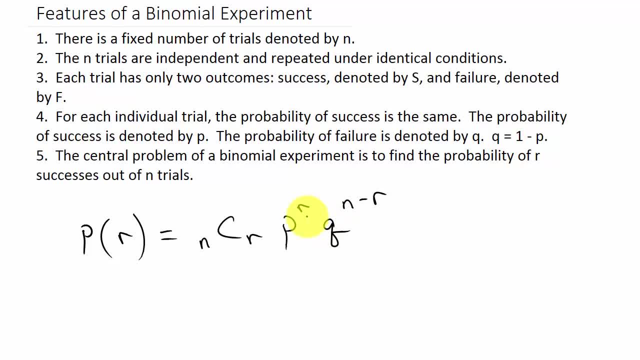 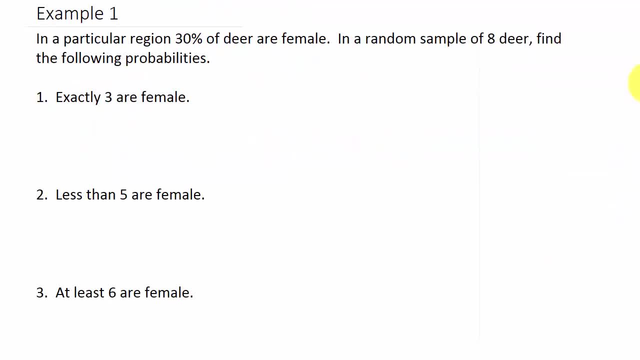 The binomial table To look up these probabilities. All right, so let's get started on our first example. All right, so it says in a particular region, 30 percent of deer are female. In a random sample of eight deer, find the following probabilities: 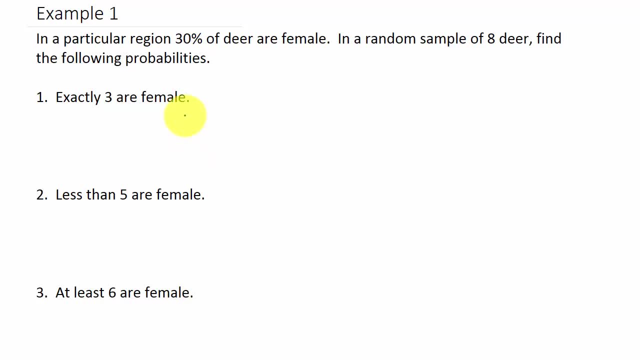 Exactly three are female. Okay, so we want to know of the. in a random sample of eight, Find the following probabilities: So we have eight deer. What's the prob? if we choose eight of them randomly, What's the probability that three of them are female? 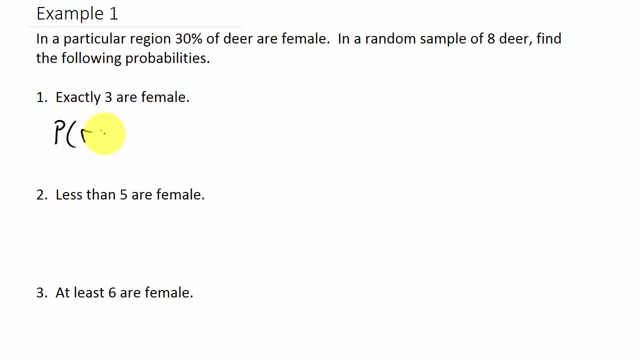 So we want to know the probability that R is equal to three. Okay, well, Remember, in our formula, Combination n, choose R Times P to the R Times Q to the n Minus R. That's the probability Of R. 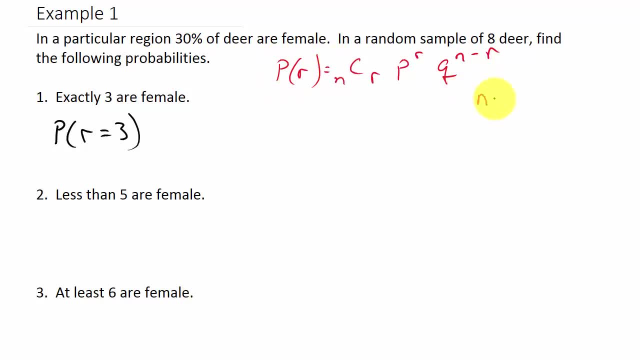 Okay, and in this case N Is equal to eight, That's the eight. P is equal to Point three. Thirty percent are female, That's point three. Q Is one minus point three, Which is point seven. Okay, 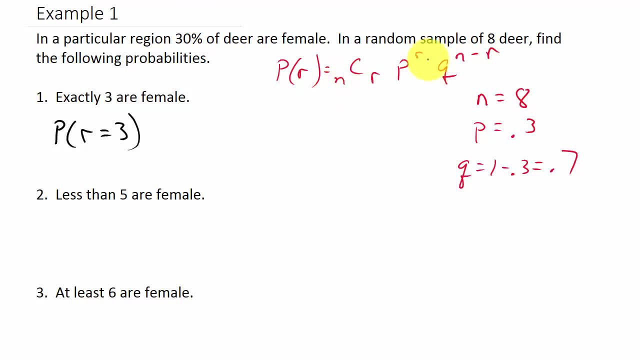 All right, So all we do now Is just plug it into this formula. So that's combination N. Choose R Times P, Which is point three, Raised to the R Times Q, Which is point seven, Raised to the n. 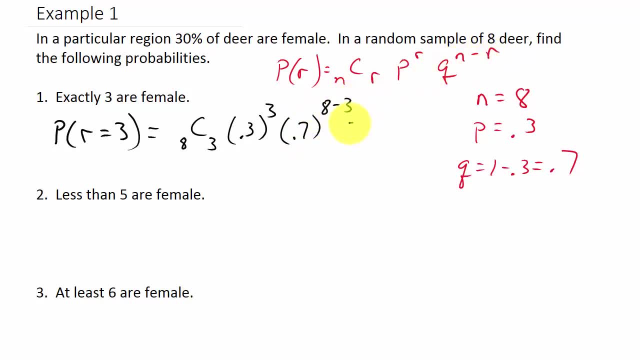 Minus R, So the eight minus three, And then you'll have to punch this Into your calculator And we get Point two, five, four, one. So that would be our probability. Okay, Now let's do the same thing here. 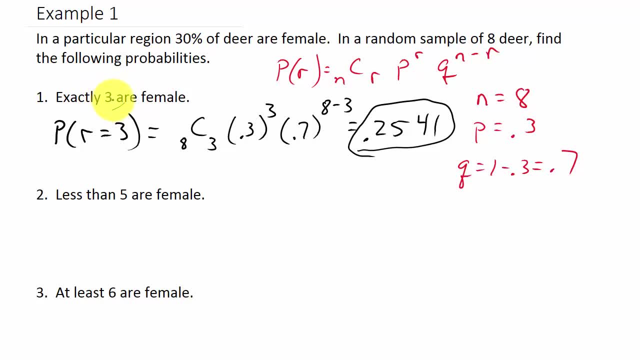 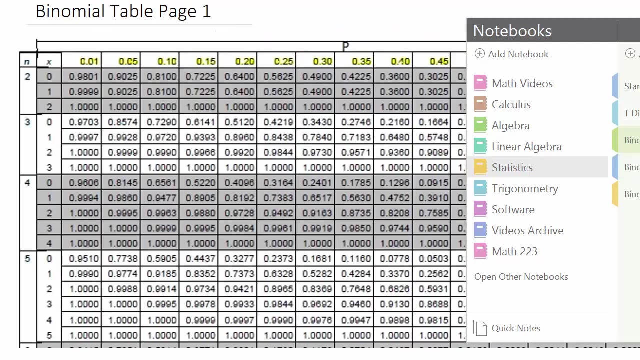 But let's look up This in the table. So remember, N is eight, P is point three And R is three. So if we come over here to our Table, Okay. So here's a table, Here's N. 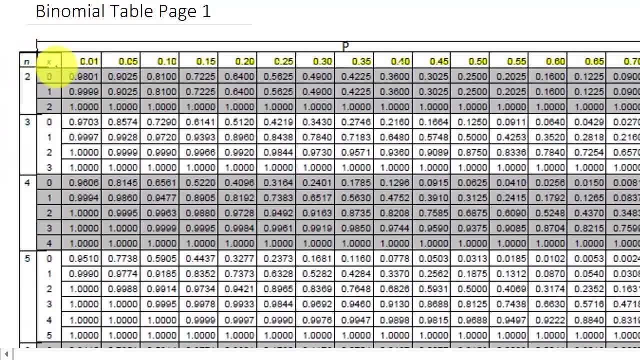 Okay, And I know on this table It has an X. here. Some books use X, Some use R. In our case, We use a R. Okay, And it's the same thing. Okay, It's no different, Okay. 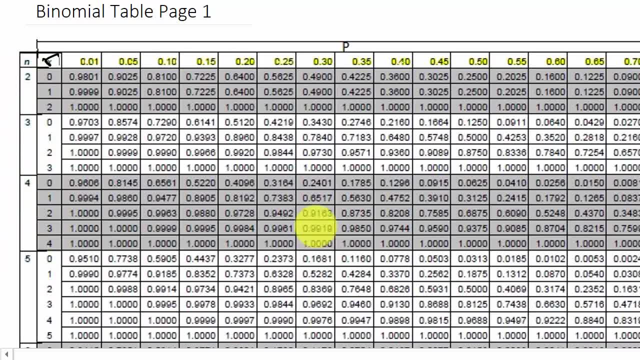 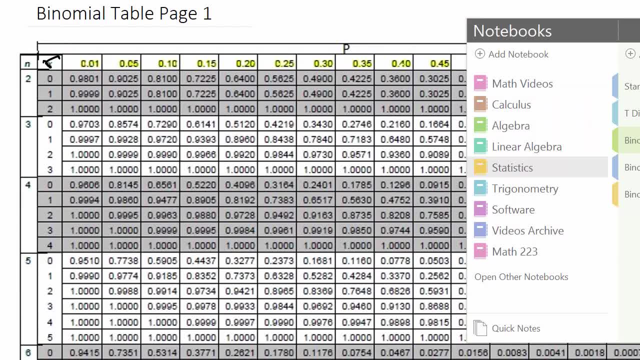 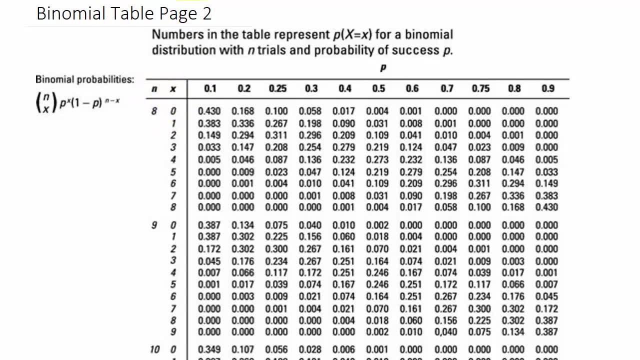 So let's look for where N is eight. Well, on this part of the table, This one just goes down to six, But we can continue on To another table, Okay, And you can see, here Is N equals eight, This right here. 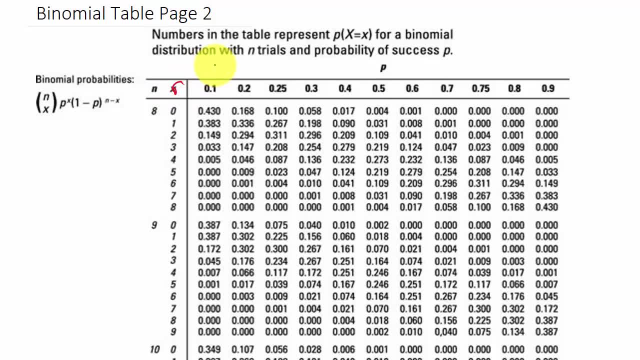 They use an X, But I'm going to use R. Okay, All right. So to look this up, We have three, Okay, And then P. This is P, This line up here. That's point three, And so you can see where. three. 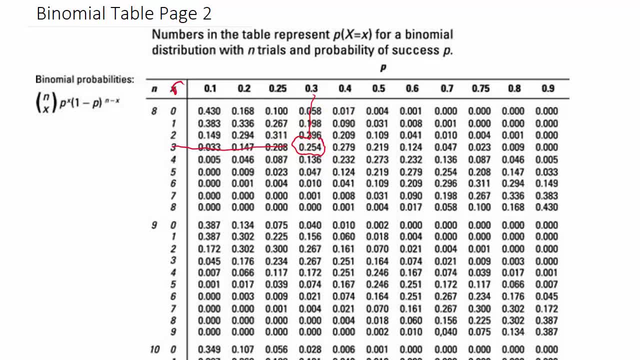 And point three Intersect. That's at point two, five, four And you can see The table rounds. it Rounds it to three decimal places. In our answer We got what point two, five, four, one. So that's using the formula. 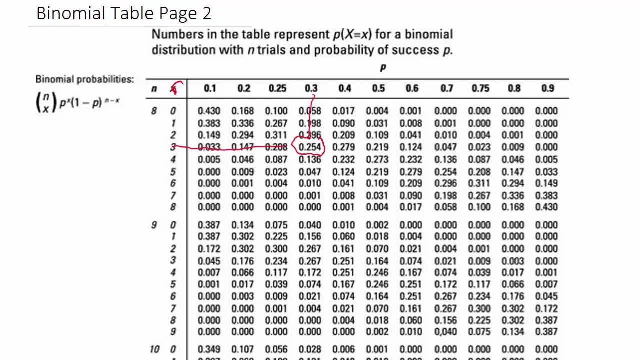 And here's using the table. Actually, the entire answer, When you plug it into the formula, Is point two, five, four, one Two one, eight, four. Okay, And from this point on We're going to use the table To find the probabilities. 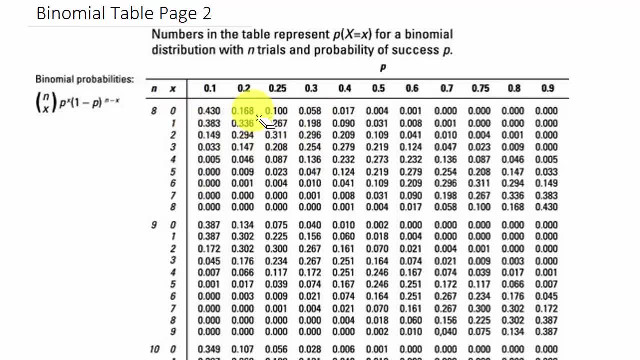 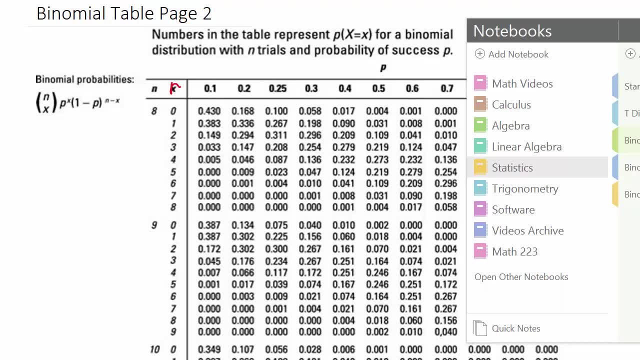 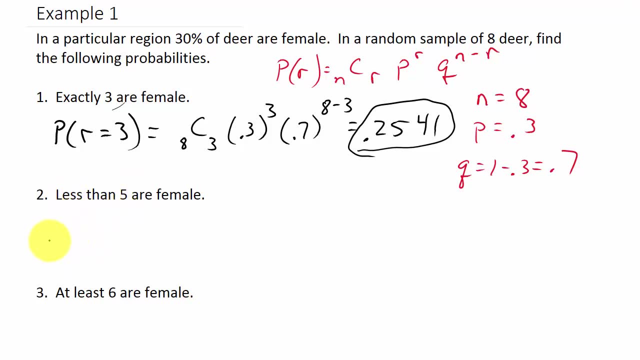 And I'll show you why in the next part of the problem. Get this Now. let's go ahead and leave the R there, Okay. So Now let's look at this one. Okay, We want to find the probability That. 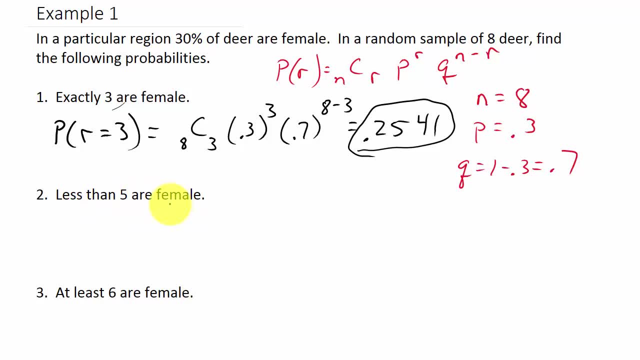 Less than five Are female. Okay, Less than five are female. So We're looking for the probability That R Is less than five. So That means That we can get zero Females, One female Or two females. 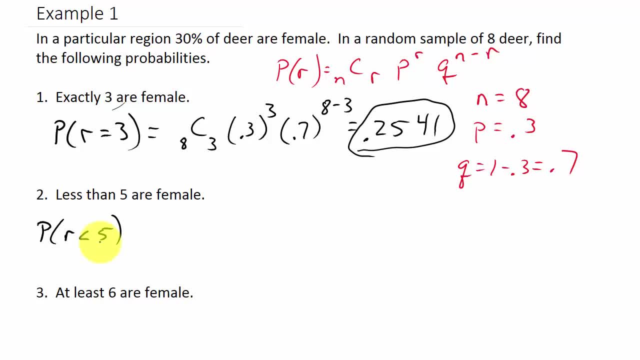 Or three females, Or four females. Okay, And let me show you why. we'll do the table instead, Because This- Now notice- the five is not included, Because it says less than five. So this is the probability of zero females. 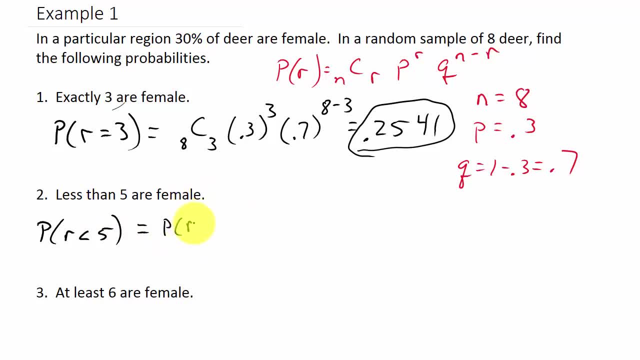 Okay, Let's go ahead and leave that in there. Or The probability Of one female, Or The probability of Two females, Or The probability of Three Females, Or The probability Of four females. Okay, 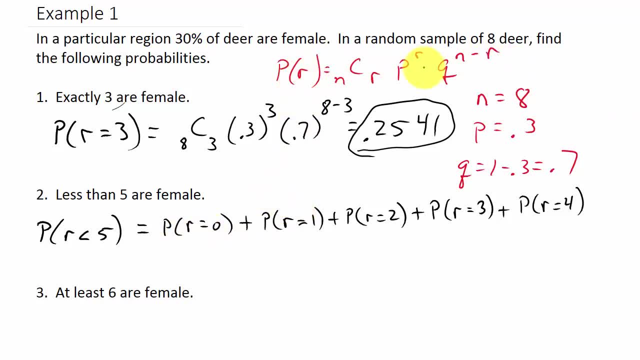 So If we use this formula up here, We would have to use this formula For each One of these. We would have to do this formula One, Two, Three, Four, Five times. Okay, So You can see how. 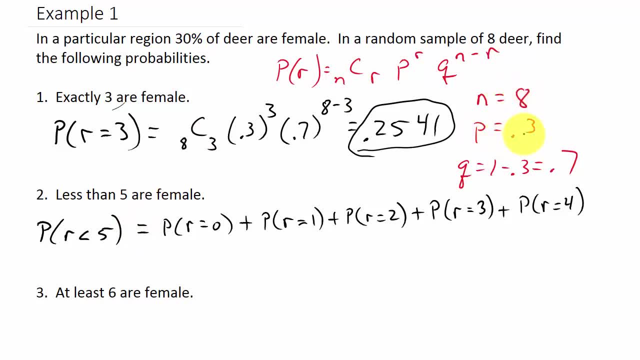 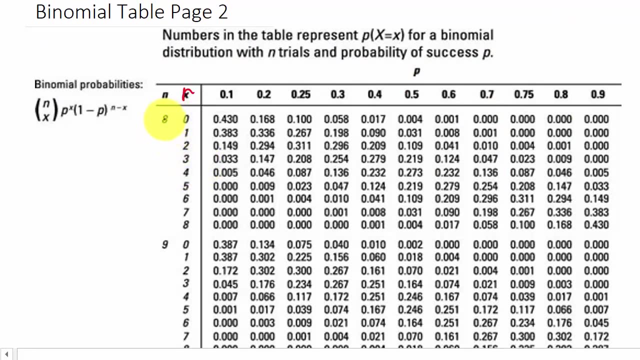 It can be kind of tedious to use the formula: Okay So We have One Two, Three Four. Okay So We have One, Two, Three Four. So That Is going to be This value when r is zero. 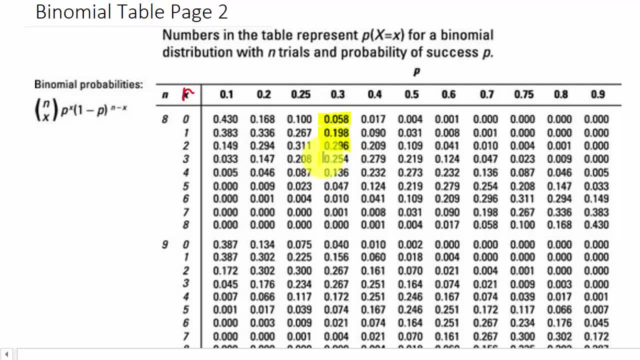 We need it when r is one, Two, Three And four. So we'll add all of these values up. Okay, So let's go ahead and write these down On the other page. Okay, So These are each one. 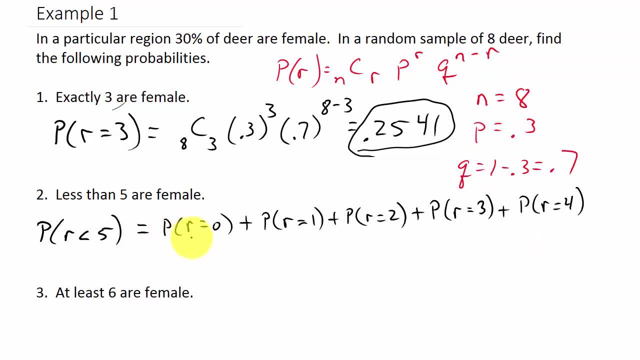 Problem. And so Remember, For r equals zero, That was point zero, five, eight Plus. And then, when r is one, Point one, nine, eight Plus. And then when r was two, Was point two, nine, six Plus. When r was three, 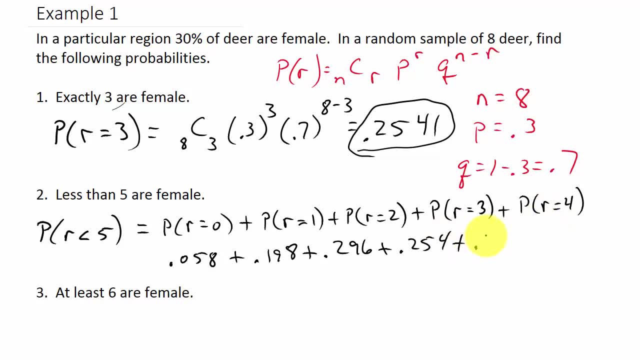 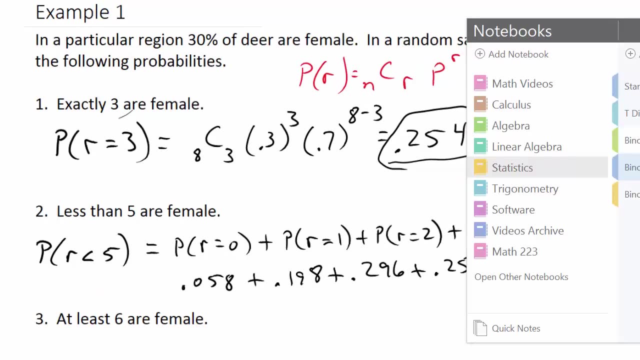 Was point two, five, four Plus Three, Six, And then we'll add all of these up And we get point nine. four. two Is our probability. Now, the other thing that I want to mention Here Is that- Let me erase this. 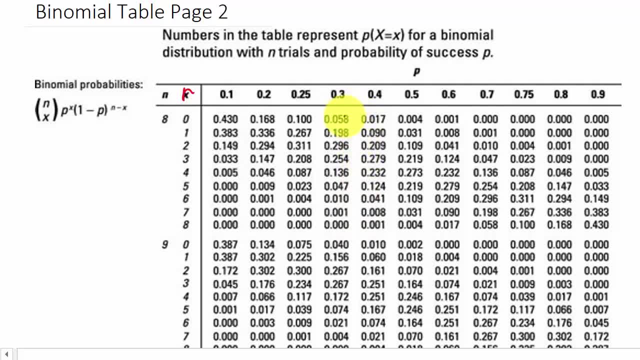 Is that? You see this little section here? All of these add up to one. Everything in this section Adds up to one. Everything in this section, All the numbers In each section, Add up to one. Okay, Alright, Now let's go to our. 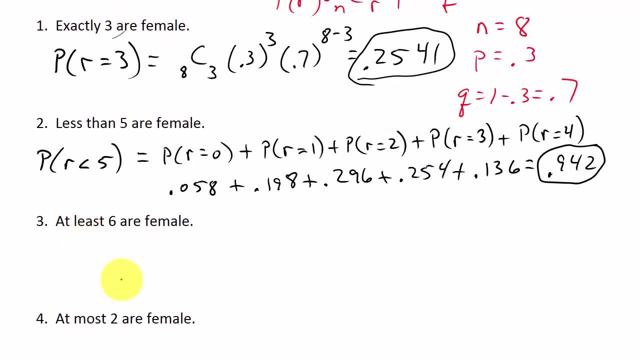 Next part. At least six are female. Okay, So at least six are female. So that means Either six Or seven Or eight are female. Okay, So the probability That r is greater than Or equal to Six. 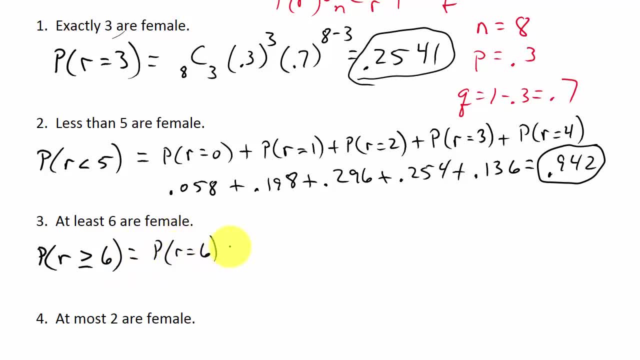 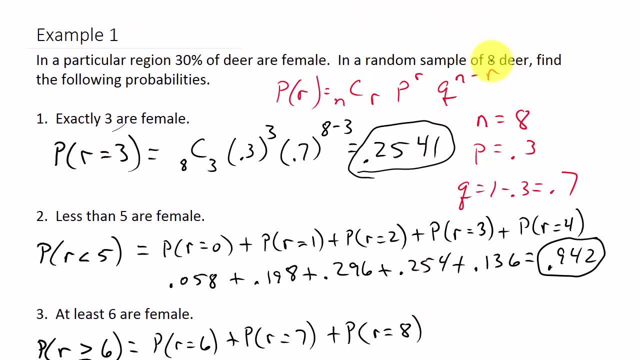 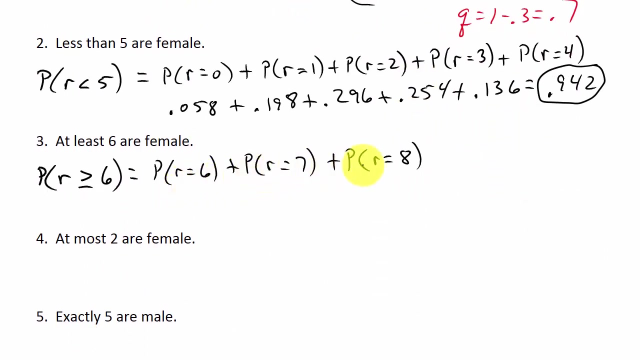 And so That's the probability That r equals six Plus the probability that r equals Seven Plus the probability that r equals Eight. See, we only go up to eight Because that's our sample Eight deer Alright, So now we'll go to the table. 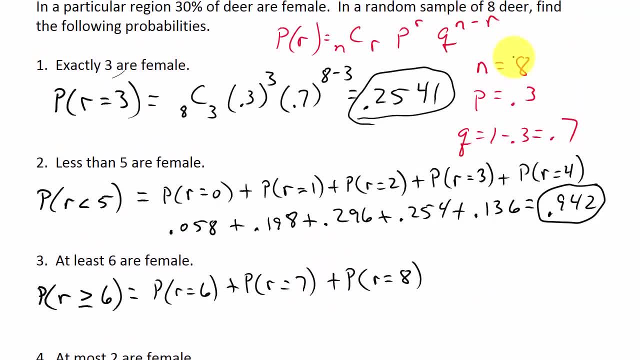 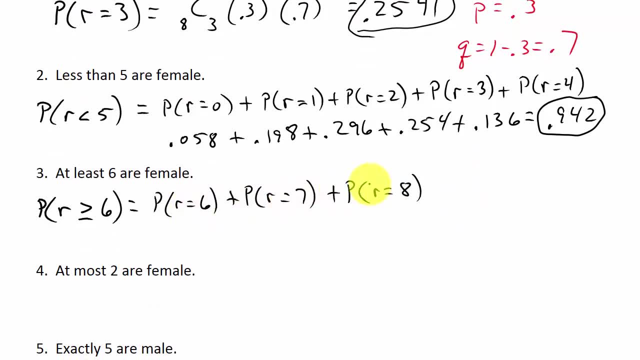 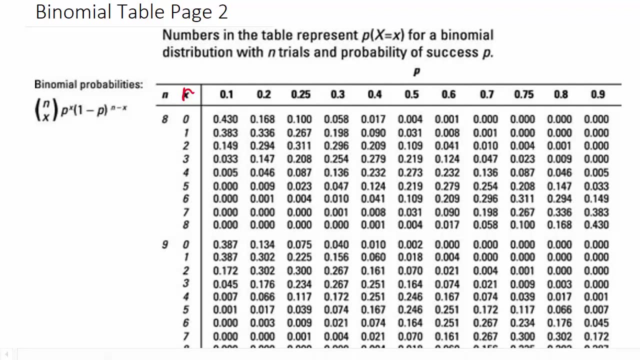 And look these up. Okay, Remember, N is eight, P is three, And we have to look them up, For r equals six, Seven And eight. Alright, So Here's: n equals eight, P equals three, And we need the probabilities. 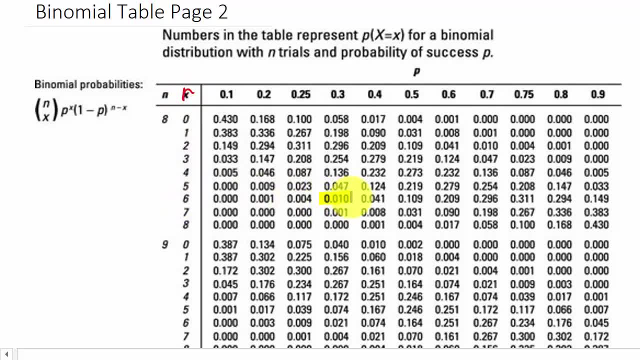 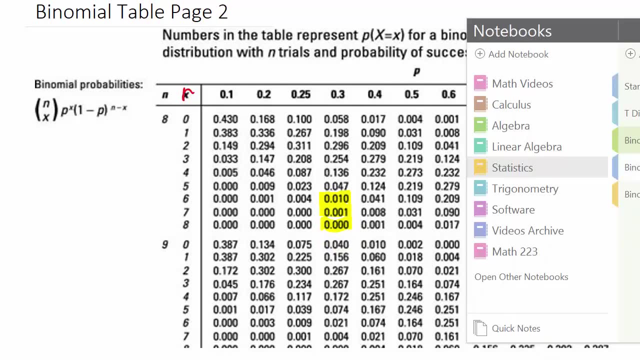 When r is six, Seven And eight, So that's point zero, one zero. Point zero, zero, one, And then point zero, zero, zero. So Let's go back to our problem. And For six That was Point zero, one, zero. 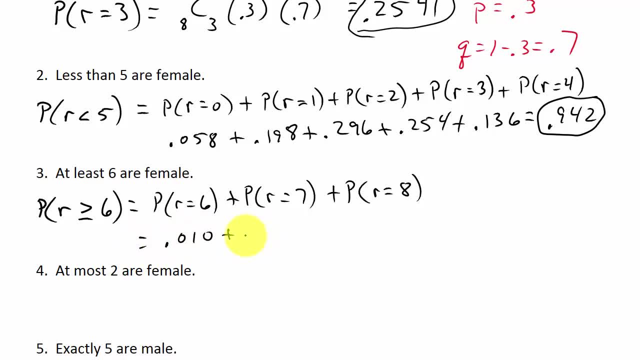 Plus, And then For the seven Point zero zero one Plus, And then the eight Point zero zero, And then When you add those together, We get Point zero one one For our answer. Okay, Alright, So let's look at the next one. 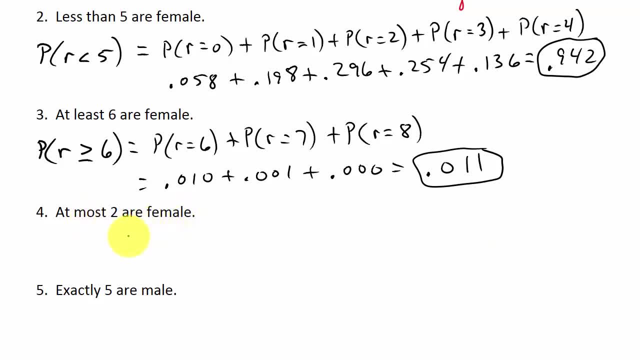 At most two are female, At most two. So that's either zero Or one Or two. Okay, The two's included here. So that's the probability That r is less than or equal to Two, So that's the probability. 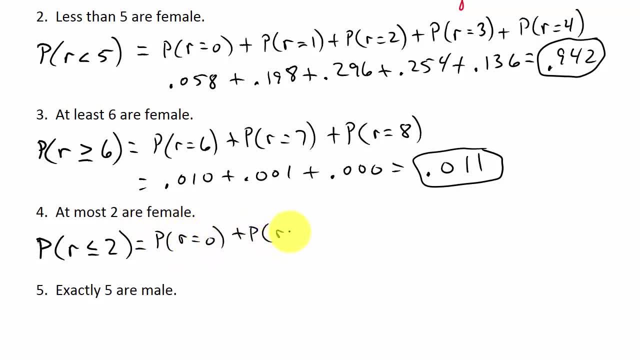 That r equals zero, Or the probability That r equals one, Or the probability That r equals two. Okay, Now We can go back to the table And look it up, But you know We've done that And I already have. 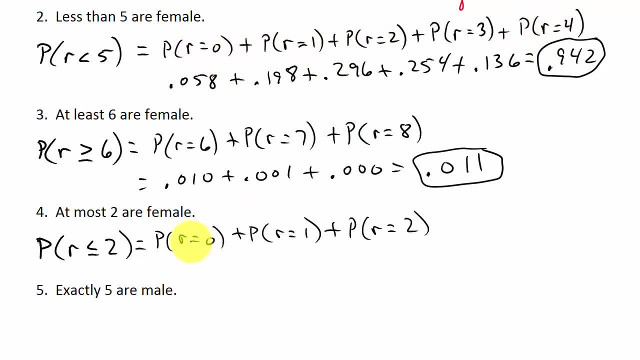 R equals zero, one and two Up here. Remember, we looked them up for this one, But this went from zero to four. We're just going from zero to two. So instead of going to the table And looking it up, Which I've already showed you how to do that- 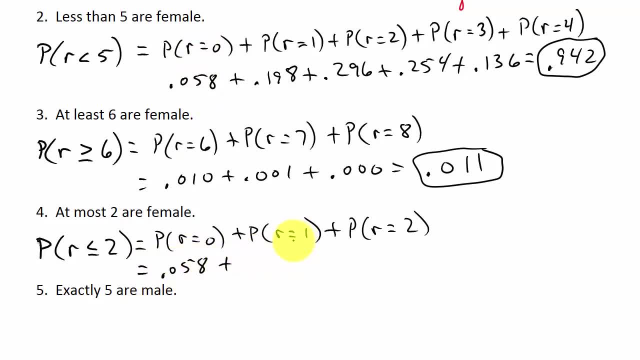 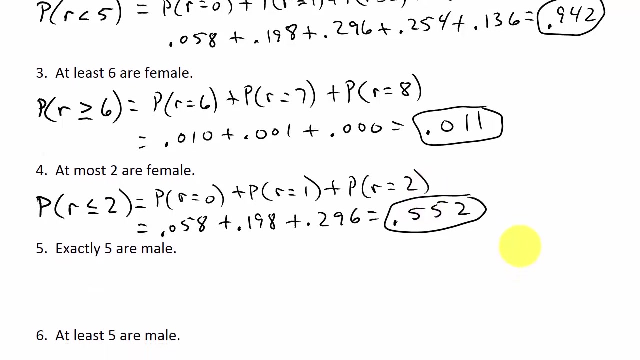 R equals zero. That's point zero. five, eight, For r equals one. That was point one. nine eight, And r equals two. Point two: nine, six, Alright, So we get point five, five, two As our probability. Alright, So now let's go to the next one. 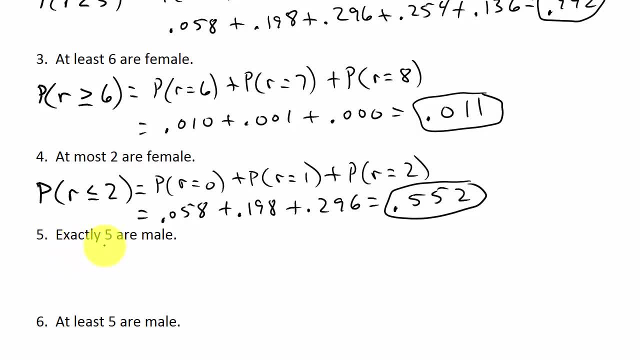 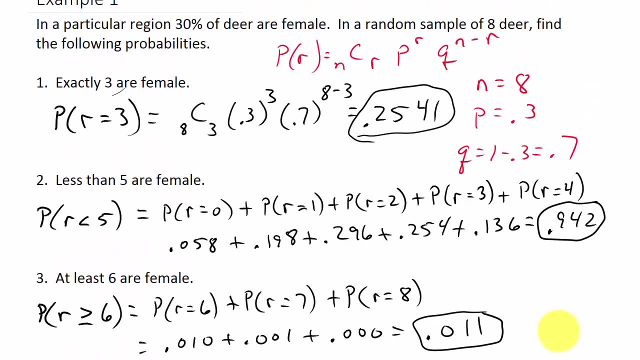 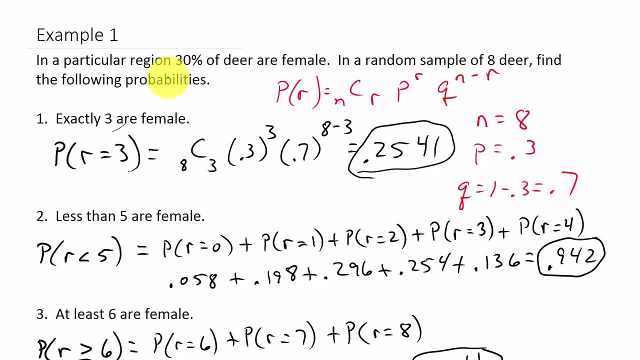 And it says Exactly five Are male. Okay, So this changes. Okay, This right here. Point three: That's the problem. Remember, P is the probability of a success. So point three Is p And p represents 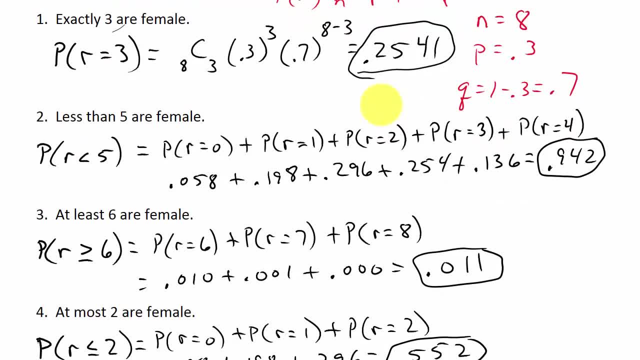 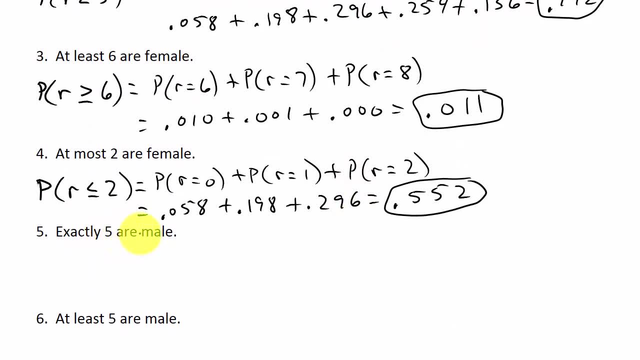 A probability of success That it's female. Okay, And p says that Are male. Well, now the probability of success Is a male. So if the probability That it's female Is point three, Then the probability That it's a male. 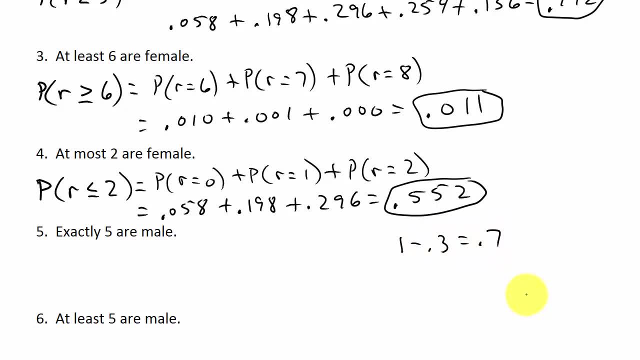 Is one minus point three, Which is point seven. So now P becomes Point seven. Okay, Because, see, our probabilities Of success has changed From female to male. So the probability That r equals Five. So we'll go back to the table. 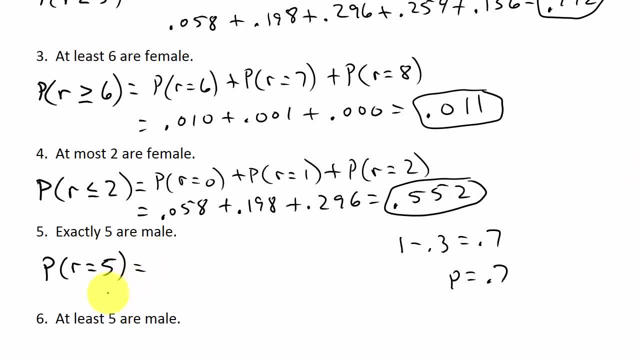 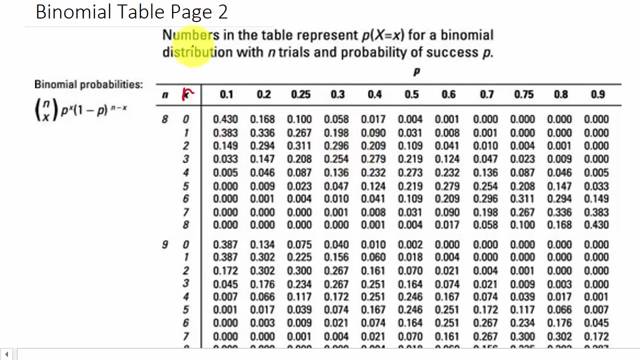 And look this, Okay, So remember, N is equal To eight, P is point seven And in this case R is five. So we'll look that up, Alright. So now We're here Where N equals, eight. 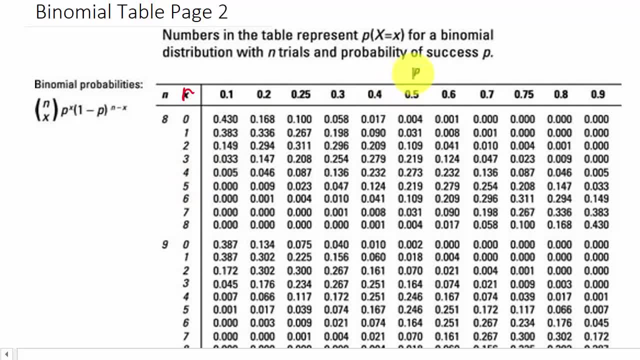 R equals five. But remember this time, Since we're finding the probability Of a male, That was point seven, So we're over here on point seven now. So if we look over here, Point seven And, I'm sorry, Five. 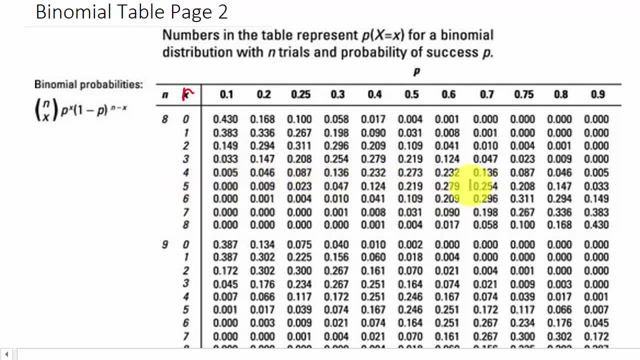 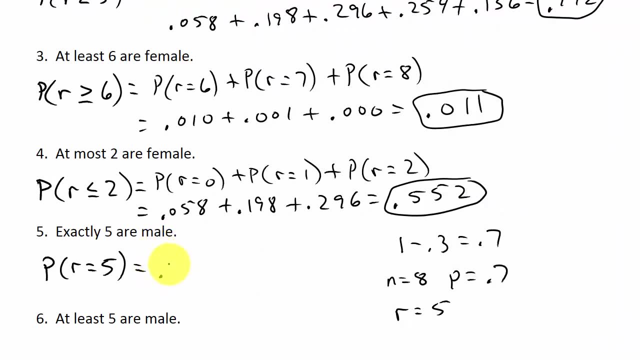 If we go over here to five And then we go to the column Where p is point seven, Our probability is this: Point two, five four. Okay, Point two, five four. So This probability Is point two five four. Alright. 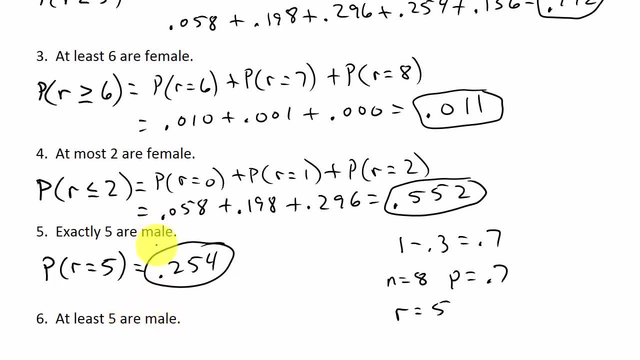 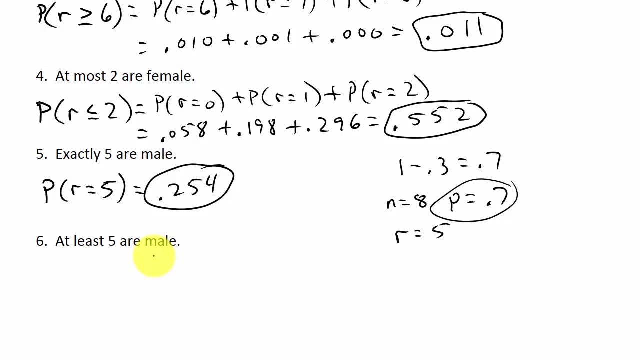 And I do have one more, But I'm not gonna do this one For the male. I just wanted to show you how the p changes, Okay, And then you know, Everything else is the same. Okay, At least five are male. 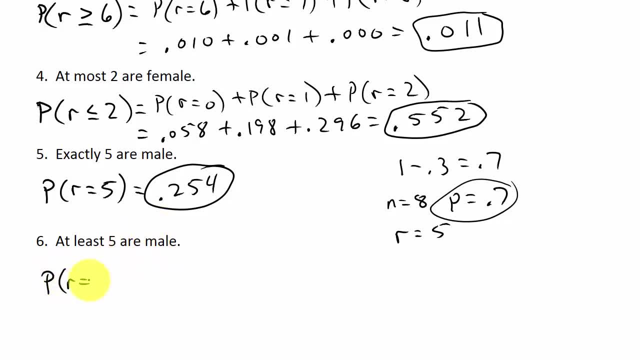 So that means five or six or seven or eight. So If we want the probability r At least five, That's r is greater than or equal to five. So that's the probability That r equals five Or the probability That r equals six. 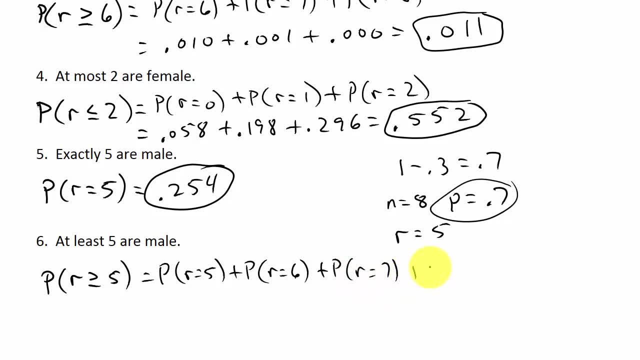 Or the probability That r equals seven, Or the probability That r equals eight. But just remember, When you go to look these up, You have to look it up in the column Where p is point seven. Okay, Just like we did for this one. 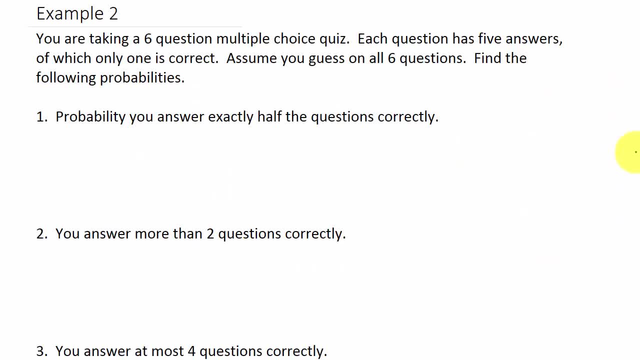 Alright, So let's go to the second problem. Alright, So Question: multiple choice quiz. Each question has five answers, Of which only one Is correct. Assume you guess on all six questions, Find the following probabilities, Probability: You answer exactly. 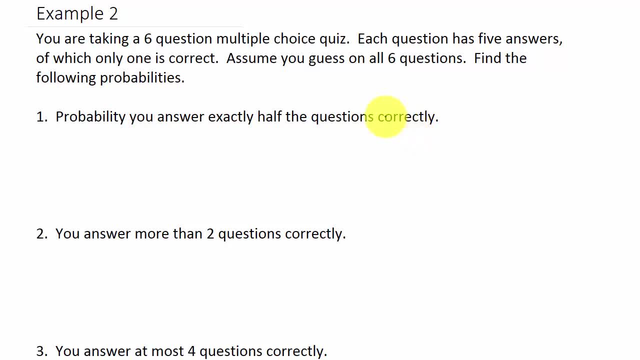 Half the questions correctly, Okay. Well, if there's six questions, Half of them would be three. So we want to know The probability That r equals three. Alright, So in this problem, N Is equal to six. There's six questions. 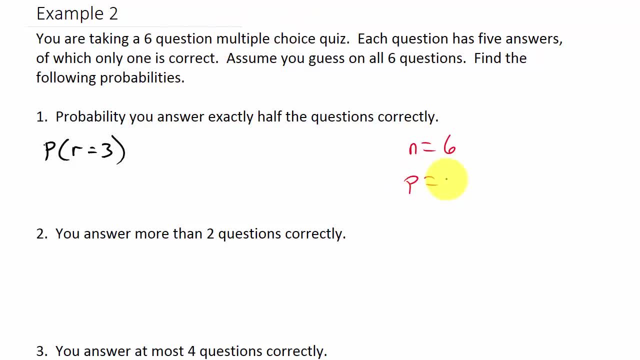 And p: Okay, Well, What's the probability of getting a question correct? Well, if there's five choices And only one's correct, Then that's one fifth, Which equals Point two, Point two. So p is point two. 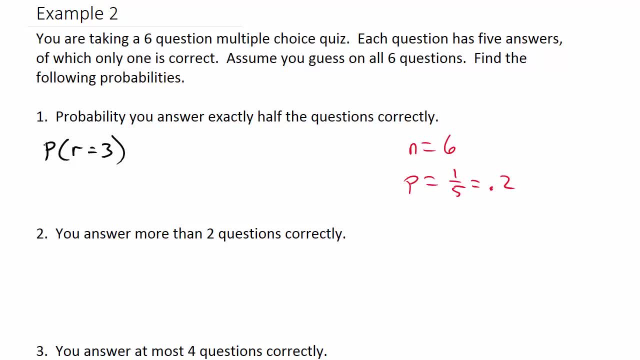 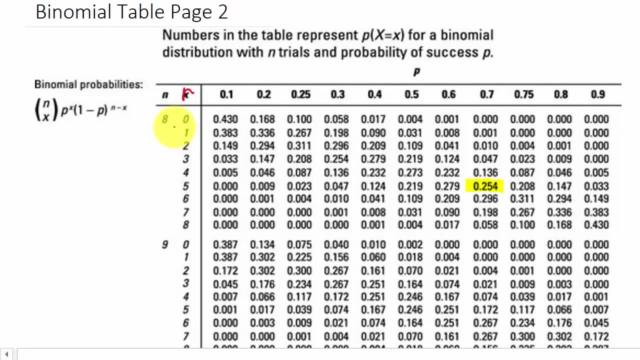 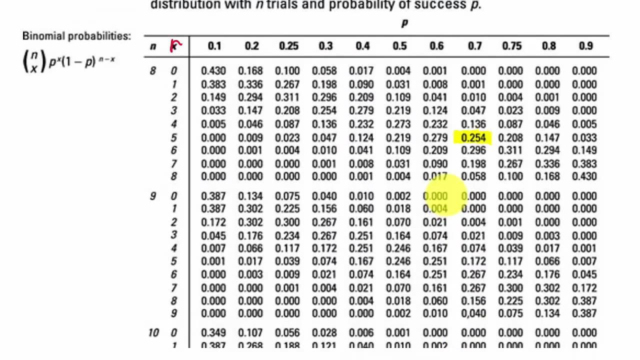 In this case, Okay. So let's go to the table And look this up, Okay, And notice this table is: N equals eight, Nine, Ten And eleven. Okay, So we'll need to go to the other page. 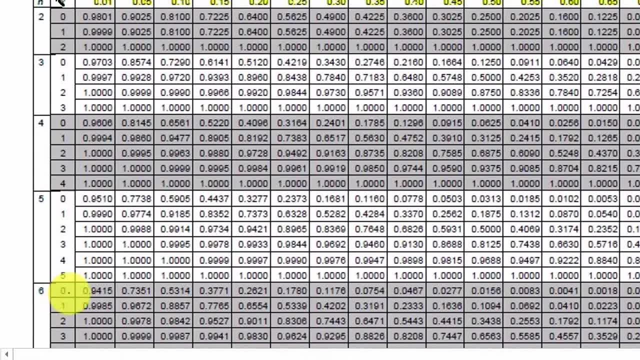 Alright. So here We're at Six. Okay, Here's r, Here's n. Okay, And we want r equals three. We need r equals three. So Here's r equals three, And we have to go to the column. 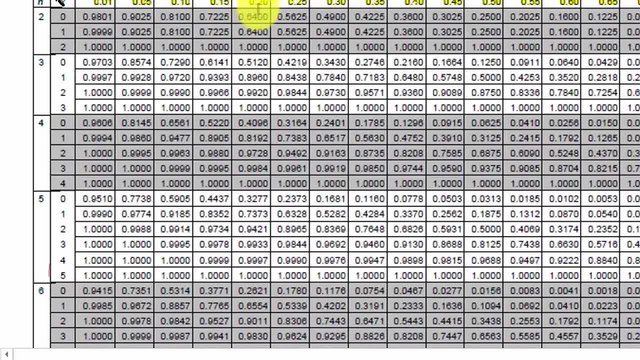 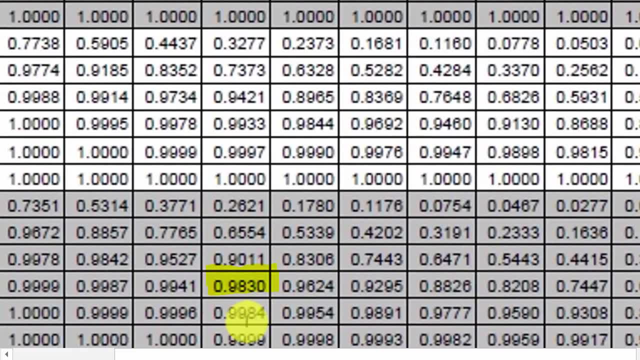 Where p, Which is this along the top, Is point two, So Three, And then we go over here to Point two. That's this value. Okay, Let me zoom it in so you can see it. So it looks like it is. 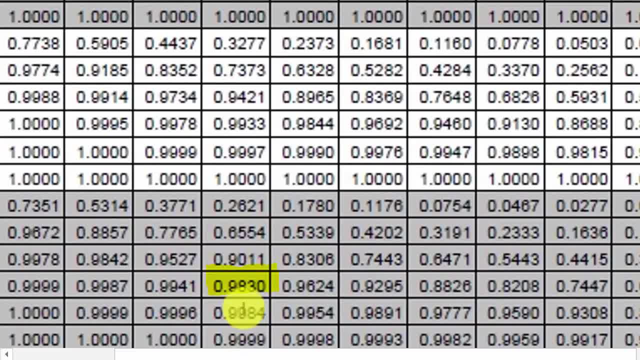 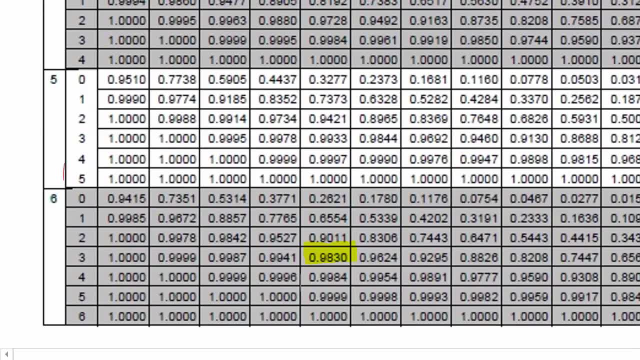 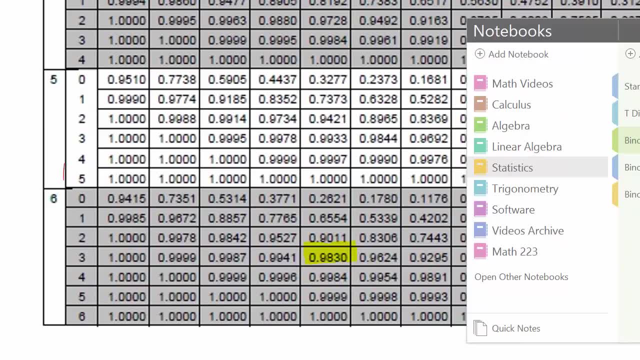 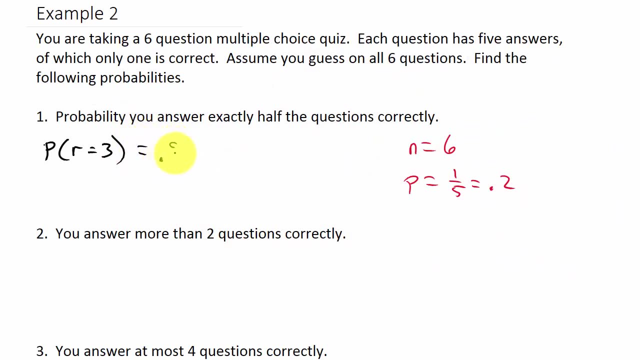 Point nine Eight Three. I guess that's what it looks like. I know it's not very, Not a very good, Not too clear, But Looks like it's point nine Eight Three. So our probability Here: 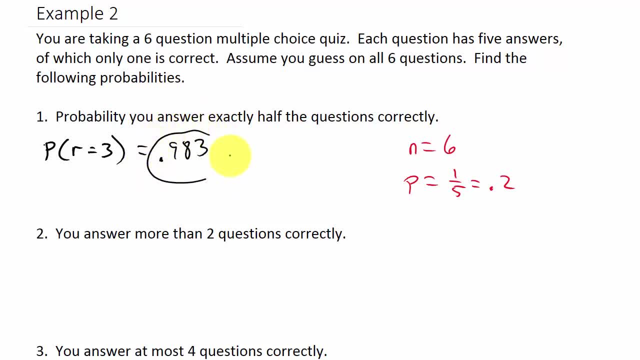 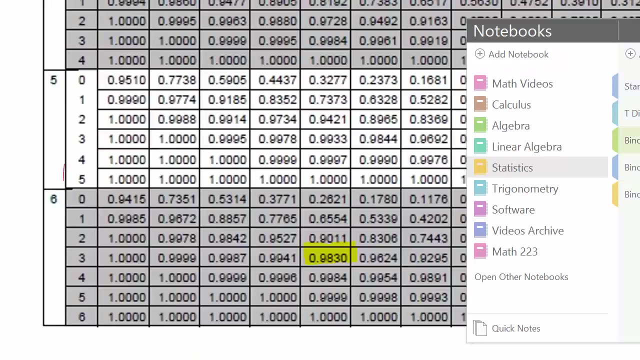 Is Point nine Eight Three, And this would be your answer. Okay, So I read the. I read the table wrong. Point Zero: Ah, Point Zero Eight Two. That's what that number should be. 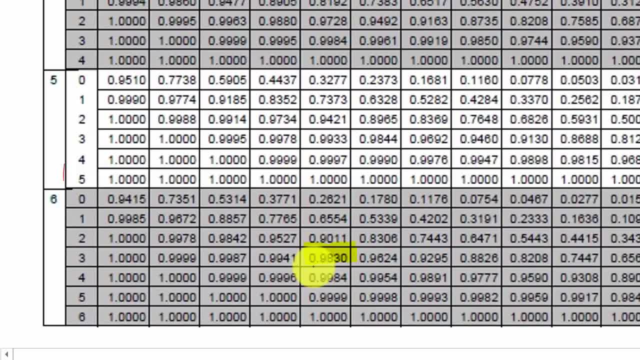 It's this number here, But it's That number is point Zero Eight, And I know this table has a three. It's a two Instead of a three, But You get the idea. Okay, I just want to make sure you know how to. 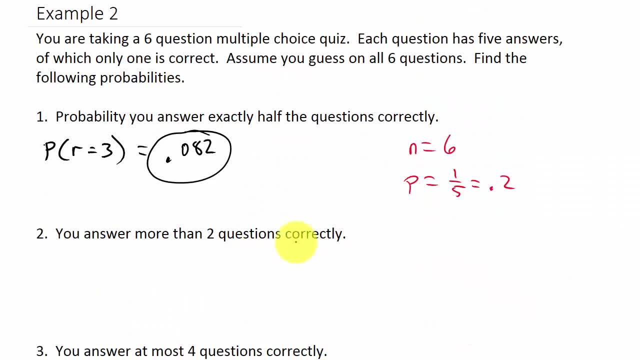 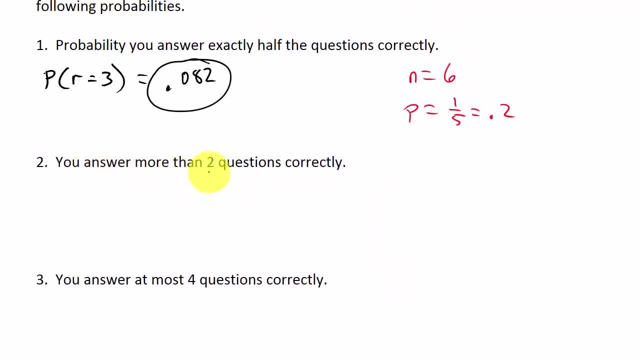 Look this up And, As far as these go, I'm not going to do these Because we're up around 22 minutes. You know how to do this. You answer more than two questions correctly. I mean we can go ahead and write it out. 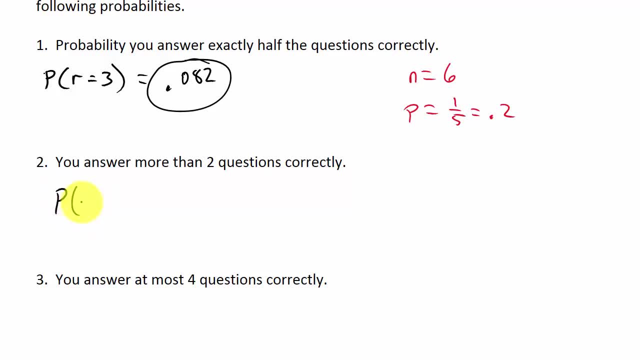 More than two questions. So that is Probability that R is greater than Two. The two is not included. Okay, So that means You're going to either get Three questions correct Or Four questions correct, Or Or. 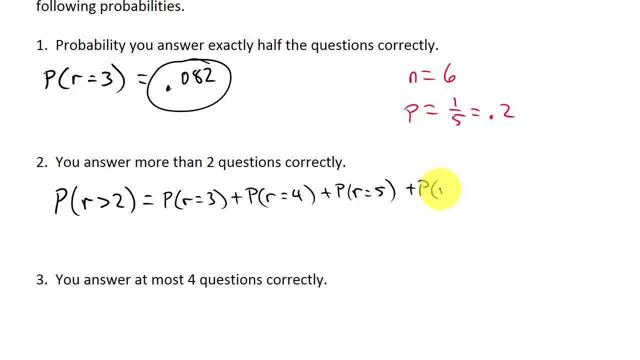 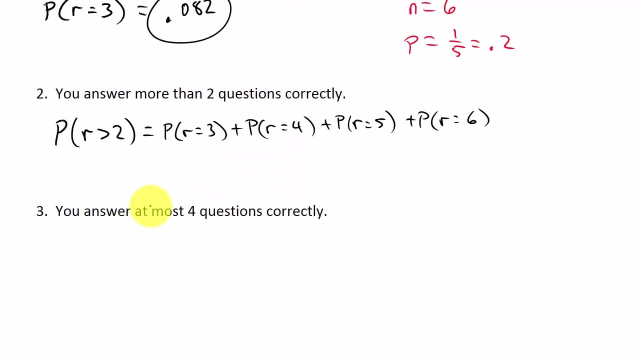 Five questions correct Or Six questions correct, And then you would go look Each of these up in the table, Where N is six And P is point two, And you would look for: R equals Three, four, five and six. 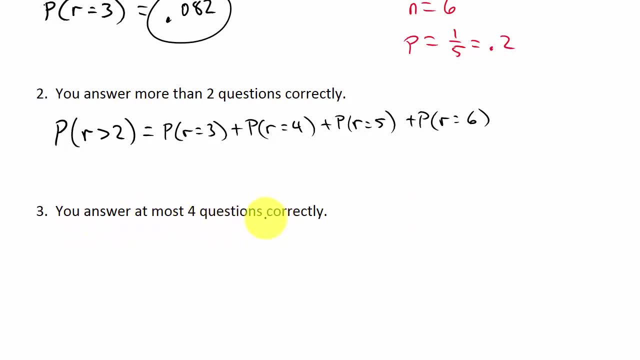 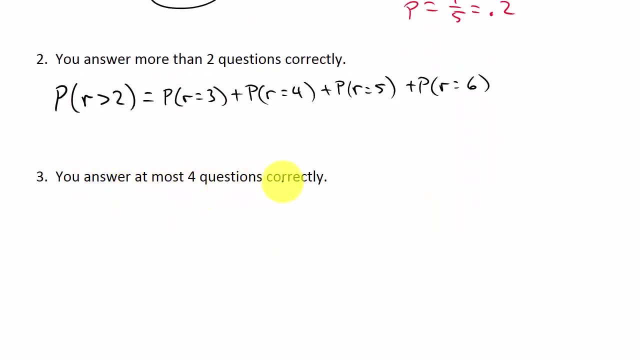 Okay. And then you answer at most Four questions correctly And see we only go up to six here, Because that's what N is Okay. So you answer at most four questions correctly. So that's the probability that R Is less than or equal to four. 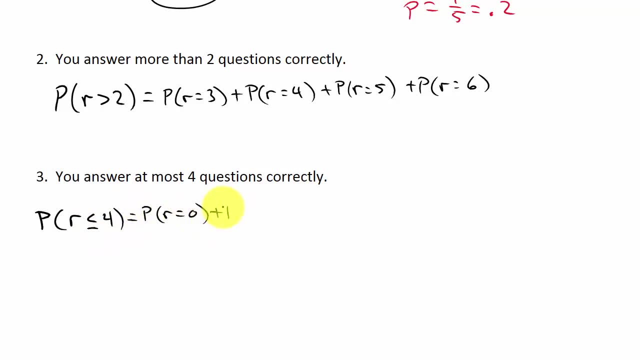 So that's R is zero questions correctly, Or One question correctly, Or Two questions correctly, Or Three questions correctly, Or Four questions correctly, And then you would look Each of these up. Okay, Alright, so I hope this video helped. 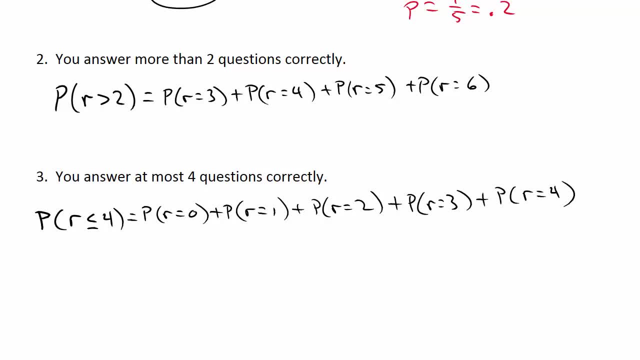 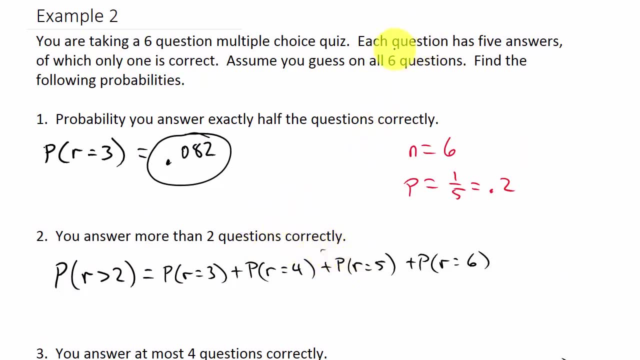 It was kind of long, But I think we covered everything. And in this last problem here, The main thing I was wanting you to see here Is, if you notice, In this problem They didn't come out and give you P Like they did in the first one.